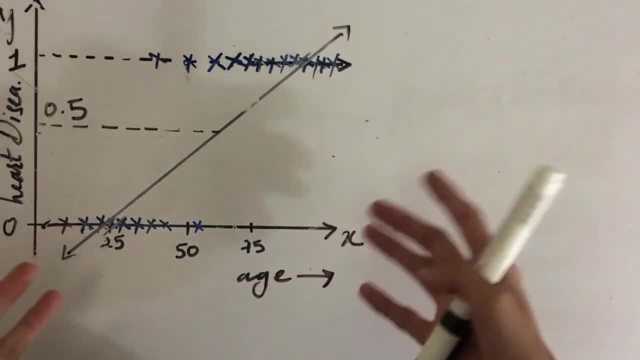 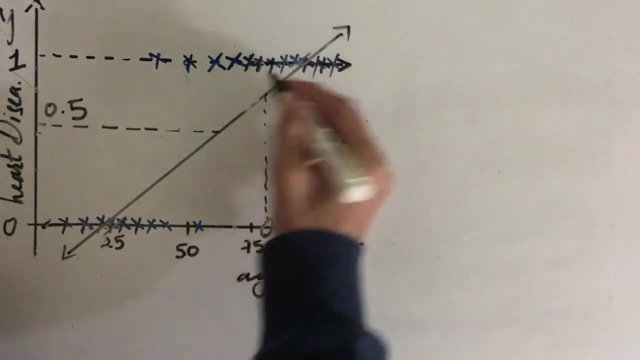 So, based on this straight line, what we can do is we can predict if the person is having a heart disease or not for a new input feature. So let's say, if we want to find if the person having this age has a heart disease or not, then what we can do is we can go to this line and see what is the. 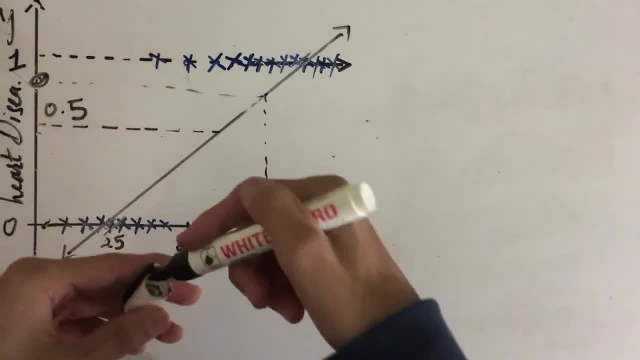 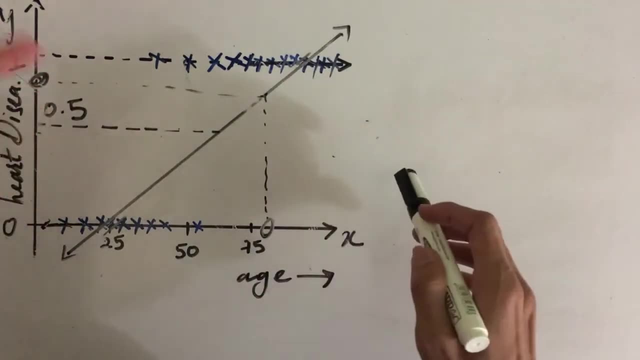 value of this. So this value will serve as the probability for us. So this is this: much is the probability that the person is having a heart disease? this probability is above 0.5, then we will classify it as 1, or if it the. 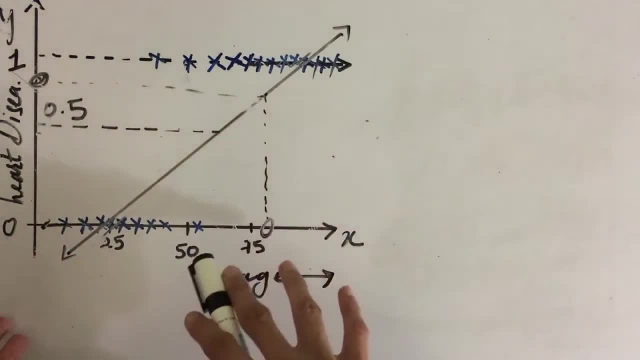 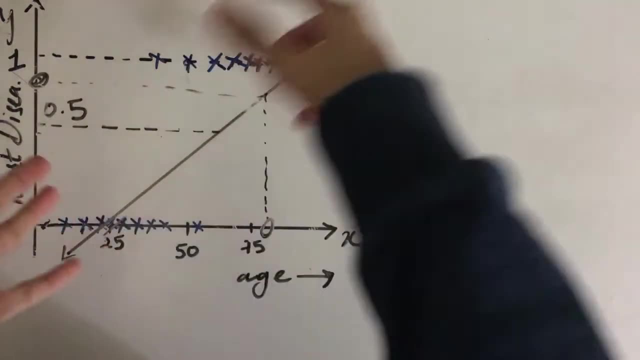 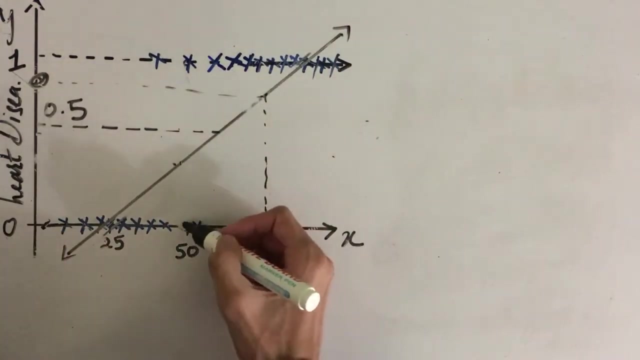 probability is below 0.5, we will classify it as 0. but this approach actually has one flaw. you can see that the straight line cannot actually fit properly to this data set. you will see a lot of gaps here, here, here, here also, let's say, if you want to predict if the person having this age has a heart. 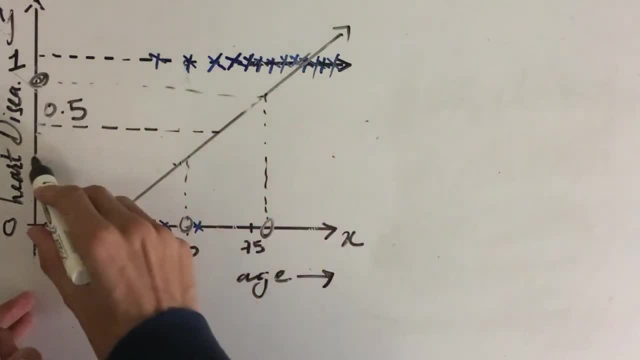 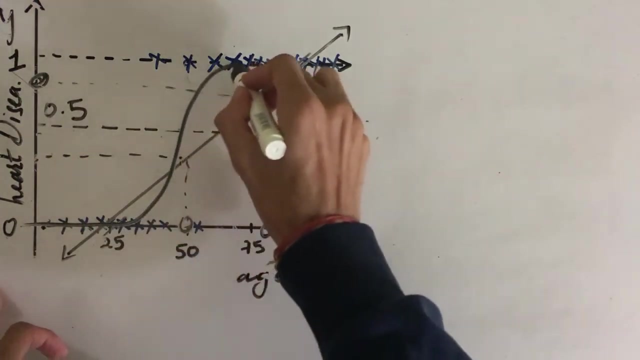 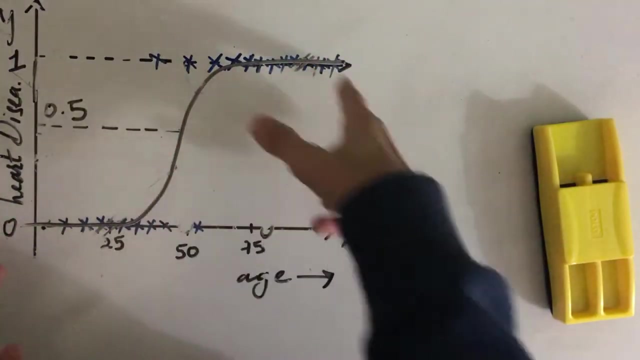 disease or not, then this method will give us actually the wrong value because it is classifying 0. so how to overcome this? one thing we can do is to draw a curve that actually fits appropriately to this data set, like this kind of curve, so you can see that this curve actually fits more appropriately to the data set. 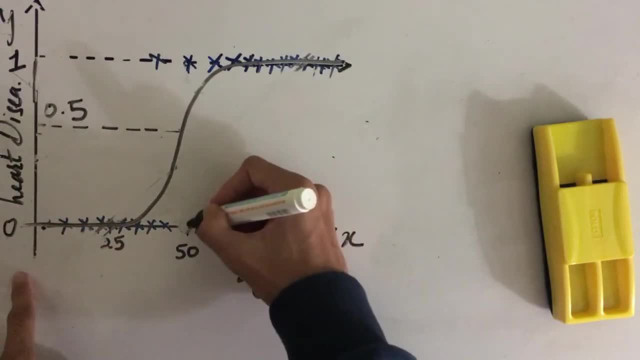 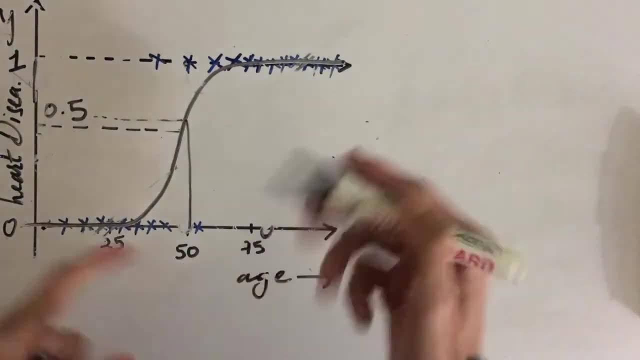 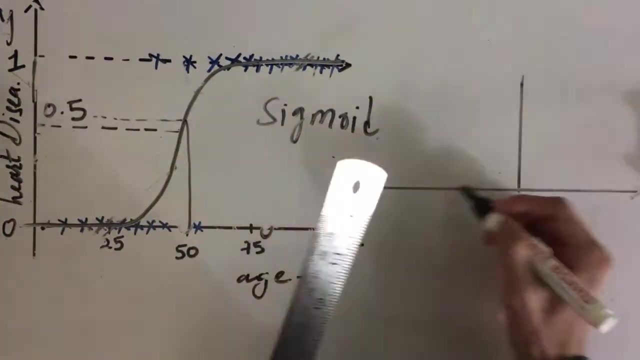 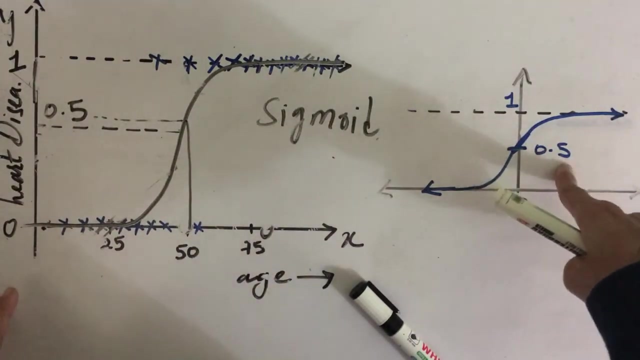 and it is also more likely to give us the right prediction. but how do we draw this curve? so this curve is actually called as sigmoid curve, and sigmoid curve look something like this: so sigmoid curves takes the 0.5 as the value when our X is 0 and when our X is. 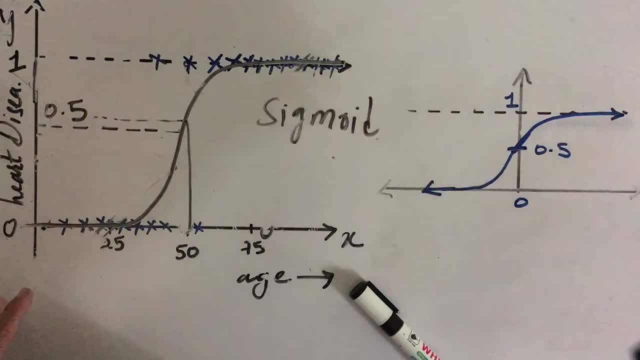 very large, it takes roughly 1 as a value- not exactly 1, but like point or so- and when the x is very low, it takes almost close to zero as the value. and the formula for this curve is 1 upon 1 plus of e power minus x. now what we can do is we can take the traditional 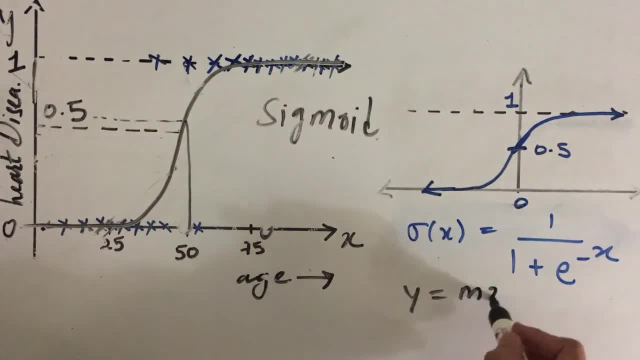 straight line that we draw with this formula y equal to mx plus c, the straight line that we draw before, and apply this straight line, a sigmoid curve. so we will just apply sigmoid of y, which will be sigmoid of mx plus c, and we will get this curve. and that's how we plot a curve that fits.